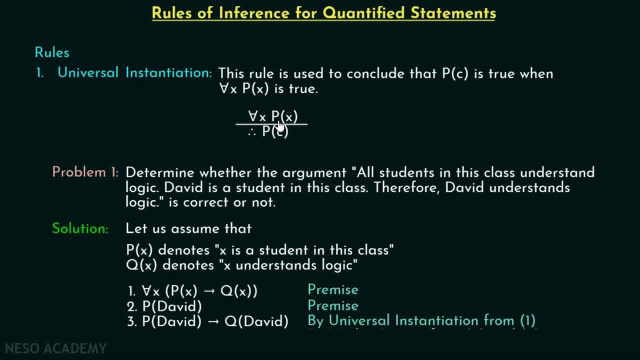 from one, because we know that if for all X PX is true, then we can also say that for some C PC has to be true. Instead of C we have David. So here we can replace this X by David, So this becomes P. 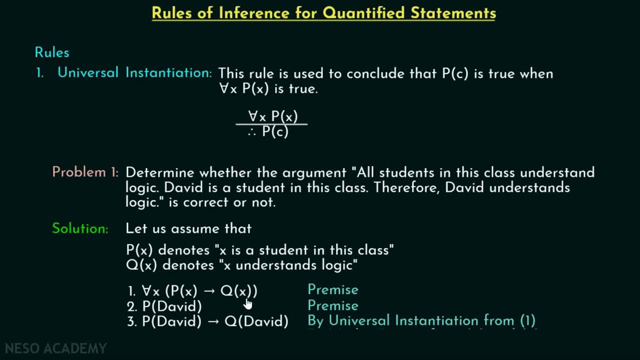 David, and we can also replace this X by David, So this becomes Q David. So we can say that P David implies Q David. by universal instantiation from one, Now from second and third we can say Q David is true. This holds true by the rule of modus ponens from second and third right. If P 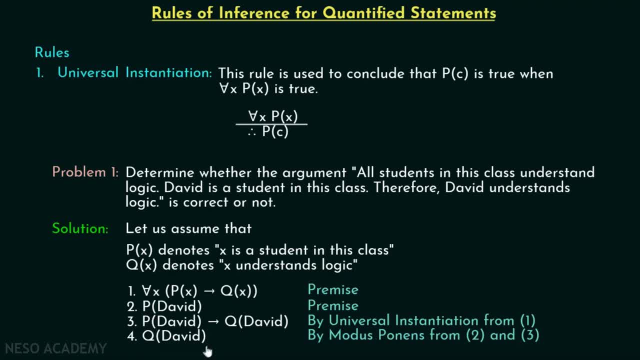 is true and P implies Q is true, then Q has to be true, Isn't that so? So Q, David, is true, which means that David understands logic. This means conclusion is derived from the set of premises, So we can say that our argument is valid. So this is the use of universal instantiation. Now, 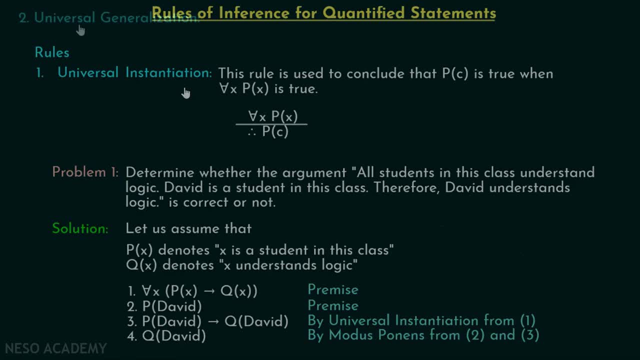 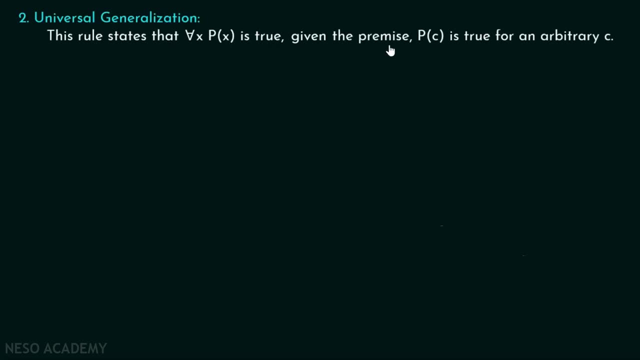 let's discuss our second rule, that is, universal generalization. So here is our second rule, that is universal generalization. This rule states that for all X, PX is true, given the premise, PC is true for an arbitrary C. Here this is opposite of what we have seen previously. Here. 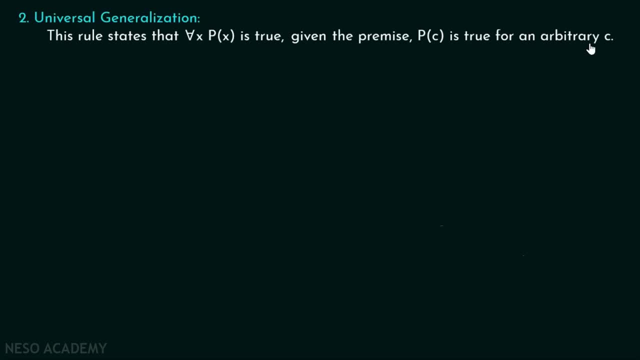 what we are saying: when PC is true for an arbitrary C, then for all X PX is true. Okay, So when PC is true for an arbitrary C, for all X PX has to be true Here. what we are considering, we are considering an 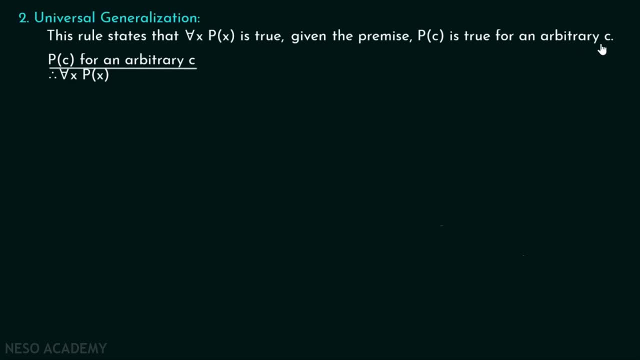 arbitrary C, That means any C We have randomly put some C inside P. If this is true, then this for all X PX has to be true. Obviously you are considering an arbitrary C, some random C, right? If for some random C PC is true, then for all X PX. 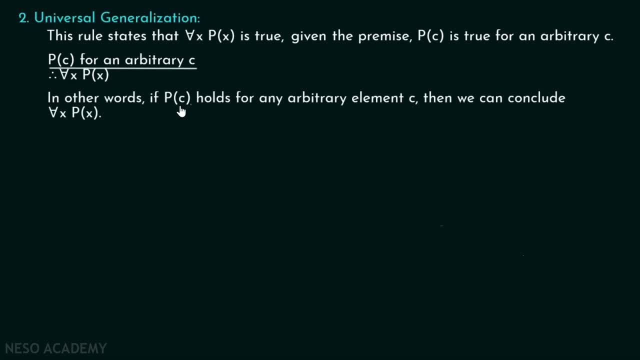 this has to be true. This is called universal generalization. In other words, we can say: if PC holds for any arbitrary element C, then we can conclude: for all X PX. Let's discuss one problem in order to understand this in a better way: Justify that if for all X PX implies QX and. 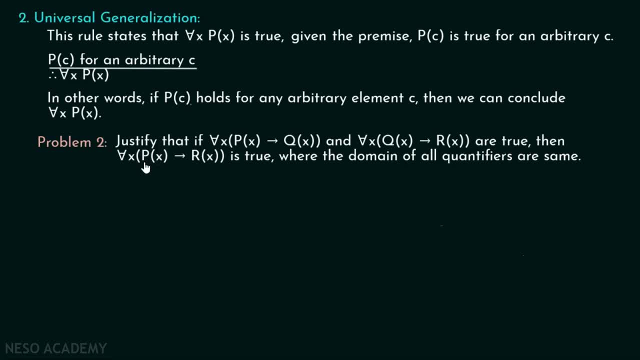 for all X, QX implies RX are true, then for all X, PX implies RX is true where the domain of all quantifiers are same. Okay, So let C be some arbitrary element Here. first we will write our first premise, that is: for all X, PX implies QX. Second premise is: for all X, QX implies RX From.